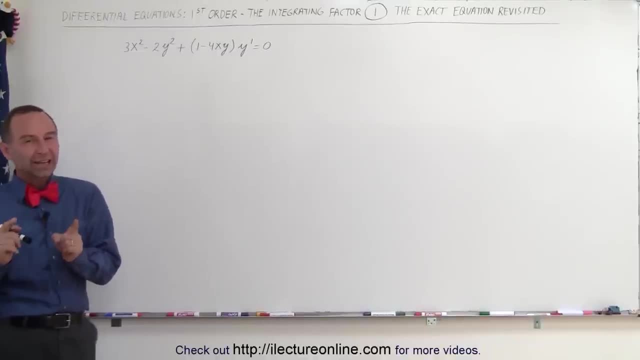 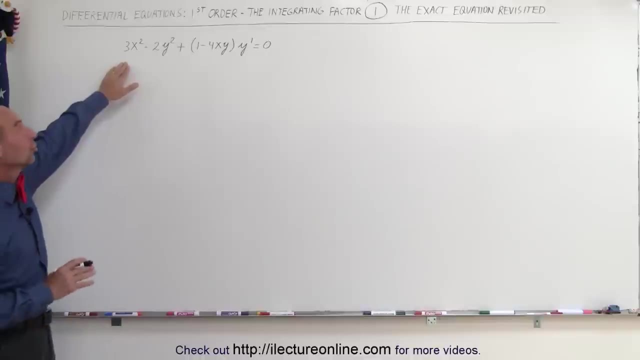 an exact equation and then we're going to show you. when the equation is not exact, you'll need in what we call an integrating factor. So here's an equation that is an exact differential equation. The left side is a vertical form. We'll show in just a moment why that is. 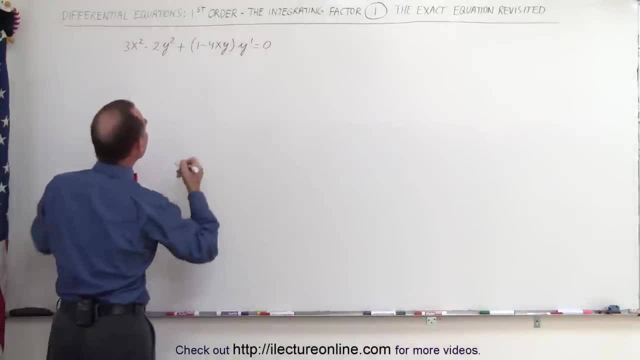 And so let's rewrite this, because y prime can be written as dy dx, So we can say that this is 3x square minus 2y square, plus the quantity 1 minus 4xy times dy dx, and that's equal to zero. Now if 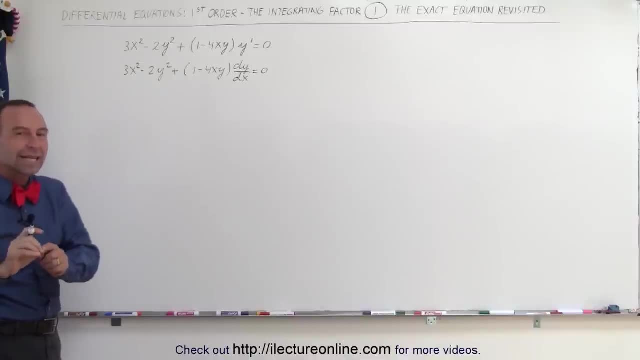 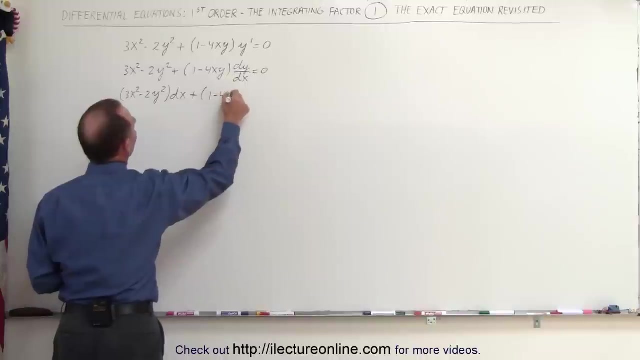 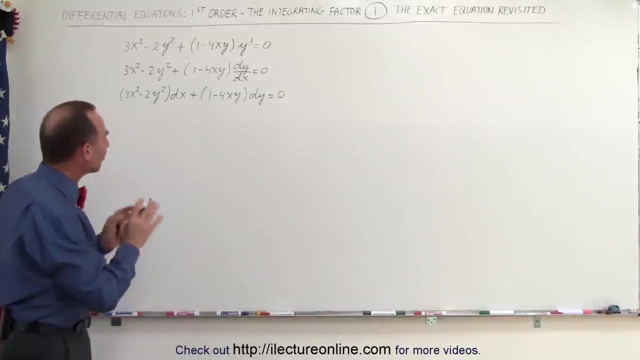 we multiply both sides by dx, we're getting the exact, in the exact form that we're looking for. So multiply both sides by dx. we get the left side to be: the quantity 3x square minus 2y square times dx plus the quantity 1 minus 4xy times dy is equal to zero. So now what that means is we have this equation in a. 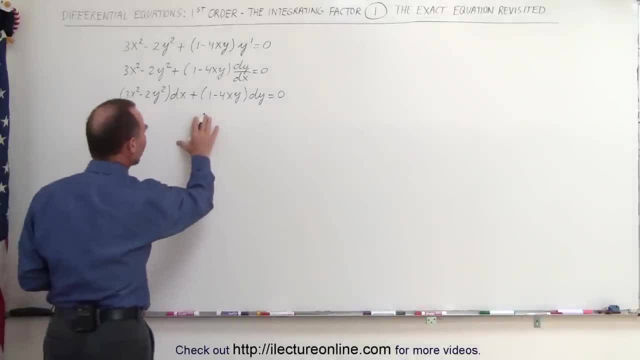 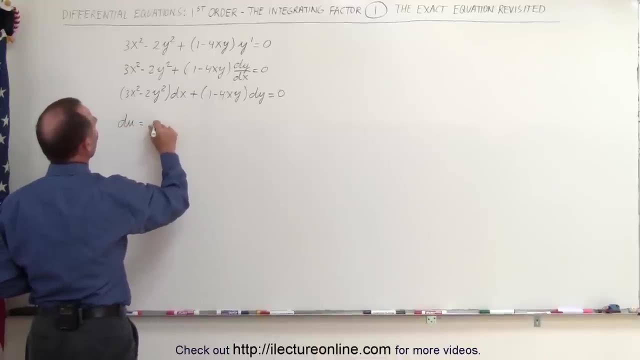 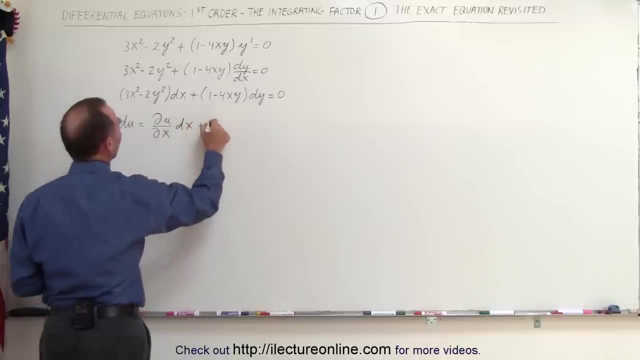 particular format, If the left side is represented by the following equation: if this cannot be written as du is equal to: and that would then be the partial derivative of u with respect to x times dx, plus the partial of u with respect to y times dy. 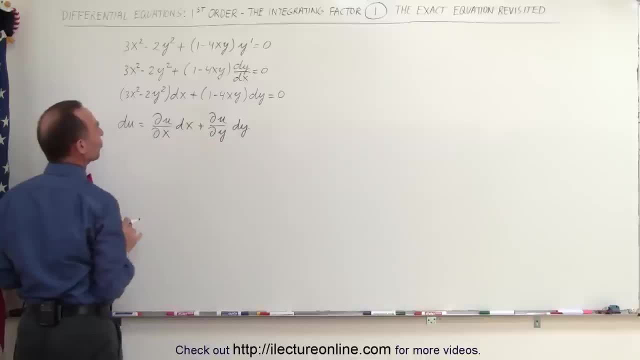 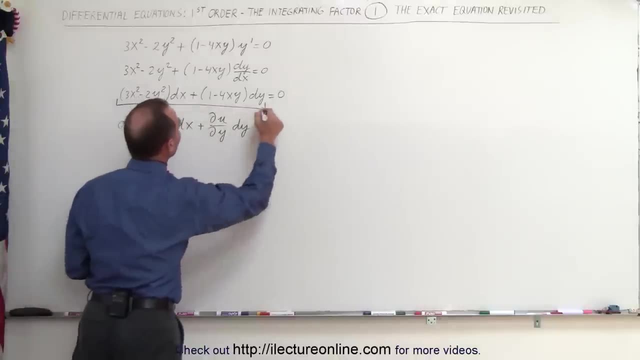 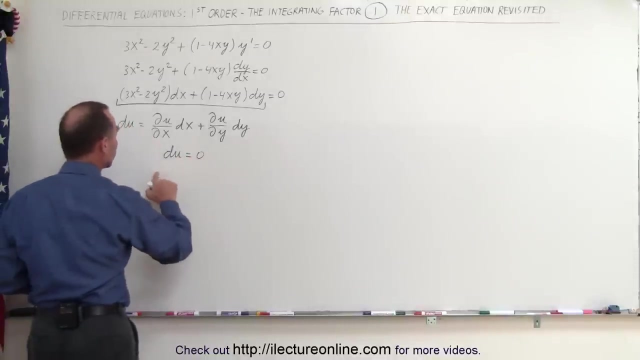 And then if we say that this is really represented by this equation right here, or at least the left side is represented by this, so then we can say that this whole left side of the equation right here can simply be written as: du is equal to zero, and then if we integrate that, we get u is equal to. 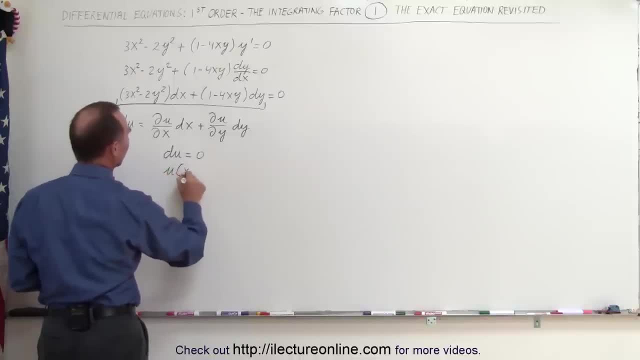 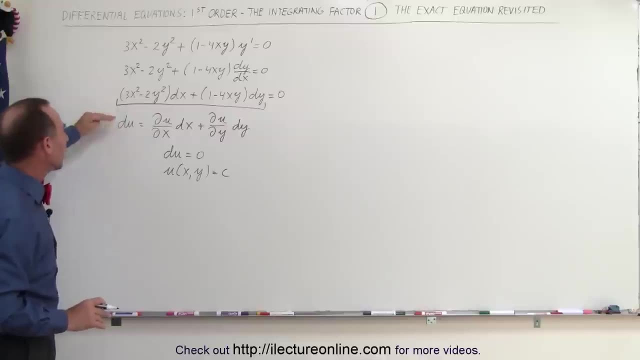 and, of course, u would be a function of x and y. it would have to be a function of x and y is equal to some constant. Now, what that means is, if this is indeed the case, if this is equal to the equation of this format, then we can say: this portion right here is equal to the partial. 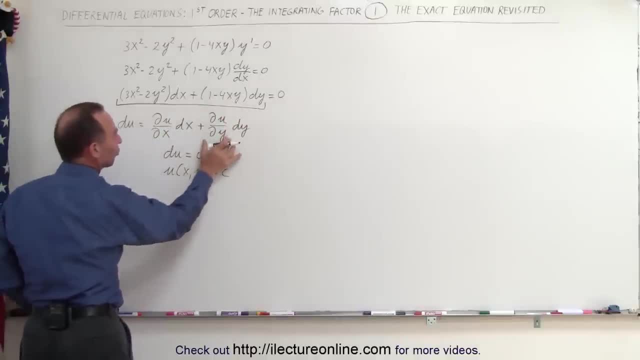 view with respect to x, this portion right here is equal to partial view with respect to y, and then we can write this equation as: m times dx plus n times dy is equal to zero, where m is equal to the partial of u, the partial of u with respect to x. 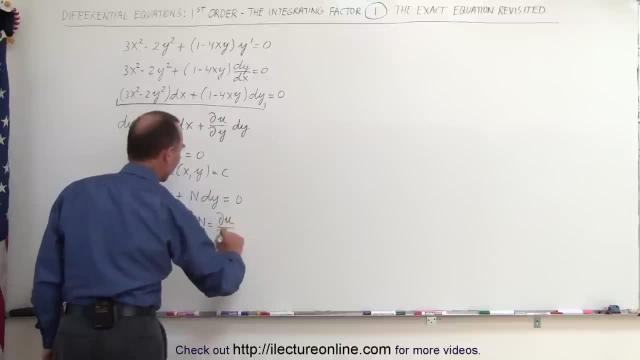 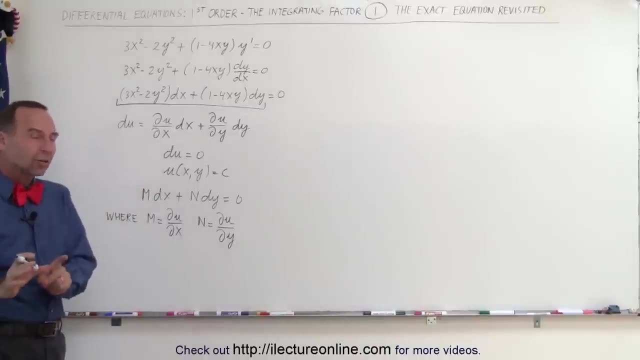 and n is equal to the partial of u with respect to y, and then if this is an exact equation- under these conditions this should be an exact equation. if it's an exact equation, we can then solve for u and then we can find the solution to this first order differential equation. 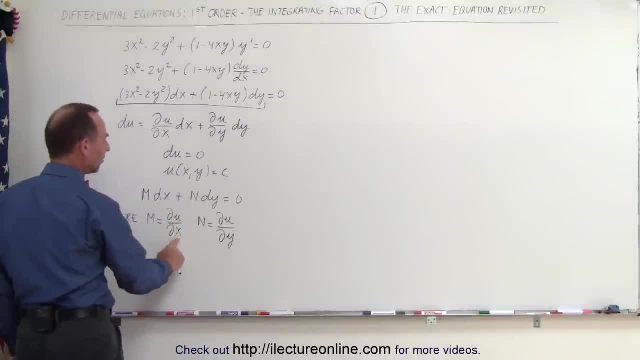 So what that means is if m is the partial of u with respect to x, and then there's the partial of u with respect to y, if we now take the partial of m with respect to y and the partial of n with respect to x, then they should be equal to one another. 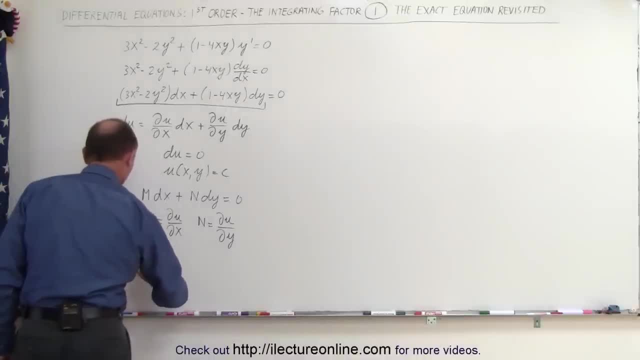 In other words, the partial of m with respect to y should equal the partial of n with respect to x, because then what you can see is that the partial of m with respect to y is really the partial of u with respect to x and respect to y, and the partial of n respect to x is equal to the partial of u with. 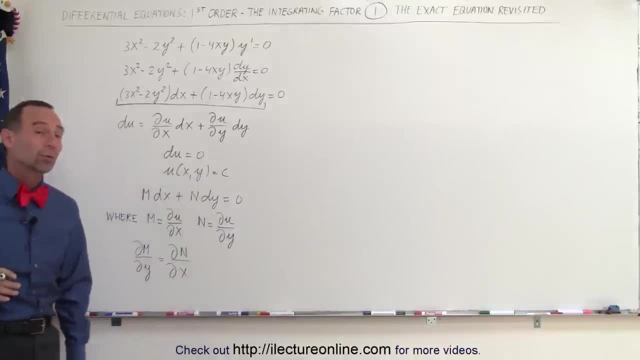 respect to y and respect to x. so therefore they must be equal to each other. and if they're equal to each other, then the equation is exact and we have a solution, or at least we can find the solution for it. what we're going to see in this series, then. if it's not an exact equation, then 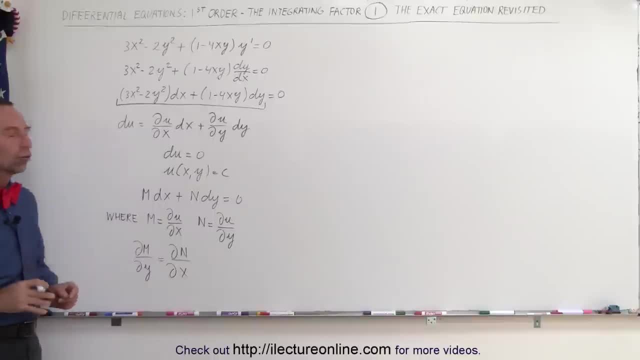 we have to use an integrating factor to make it exact so we can find the solution so quickly. to show you that this is an exact equation, we're going to take m, which is this quantity right here, and n, which is this quantity right here. take the partial respect to y. take the partial respect to x. 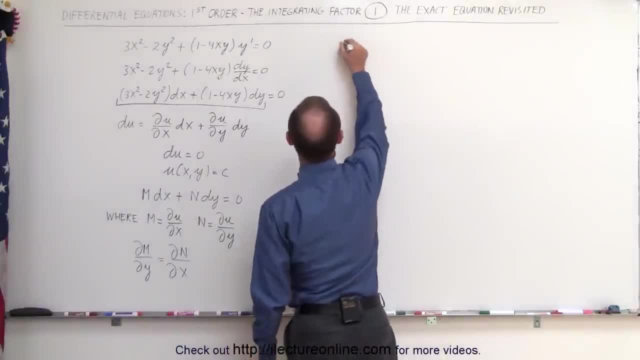 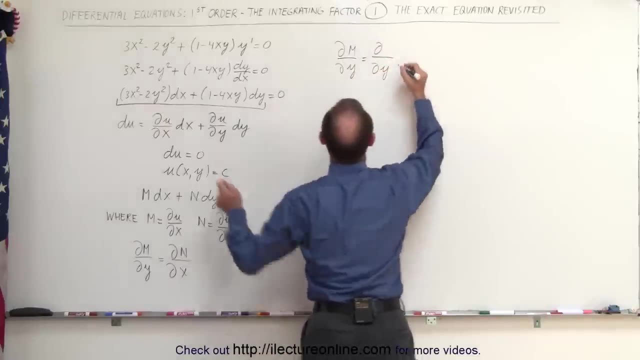 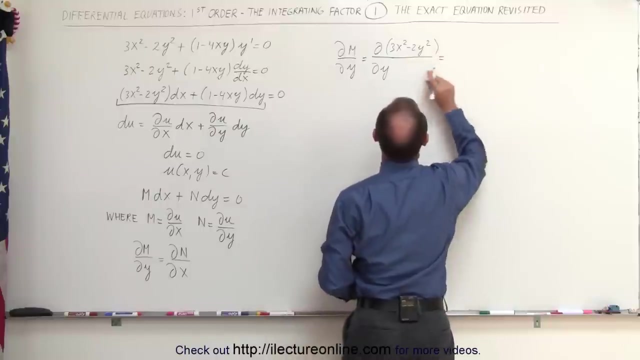 and we'll show you that they're equal to each other. so the partial of m with respect to y is the same as the partial with respect to y of this quantity right here, which is equal to 3 x squared minus 2 y squared. let's go ahead and do that real quick. so this is equal to: since x is a constant in. 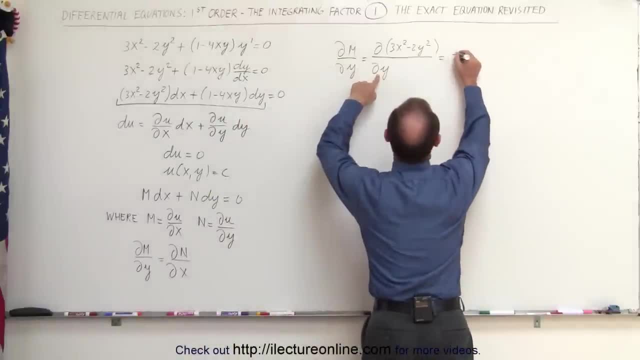 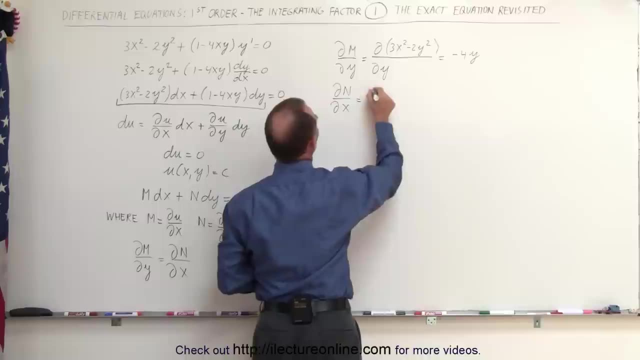 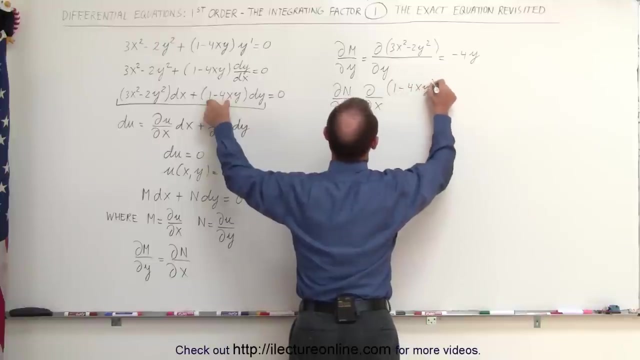 this case only y is the variable, then this would become minus 4y, and then if we take the partial of to x, this is equal to the partial, with respect to x, of the quantity right here: 1 minus 4 x, y. so this is equal. to remember: in this case y is a constant, only x is a variable, and so in this case, 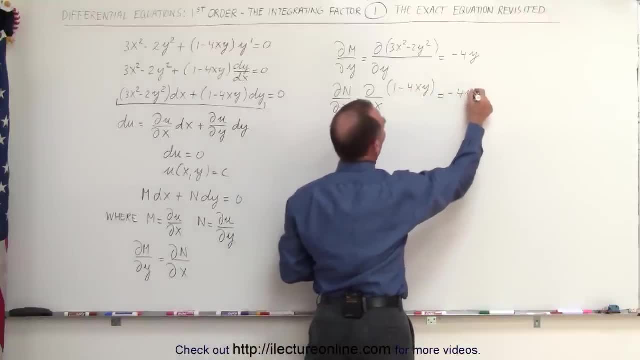 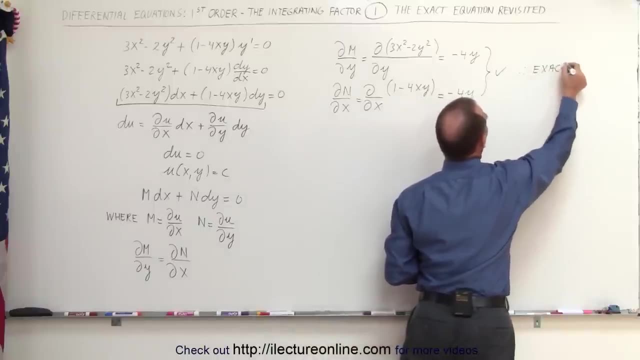 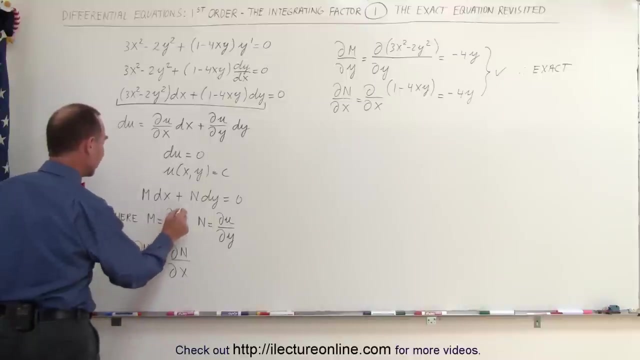 the that would be minus 4 y- and notice that these are equal to each other. so therefore, we can say: this is an exact equation. and then, if it's an exact equation, well, we'll solve it as follows. what we can say then is: we can go back over here and notice that this relationship, we can use this. 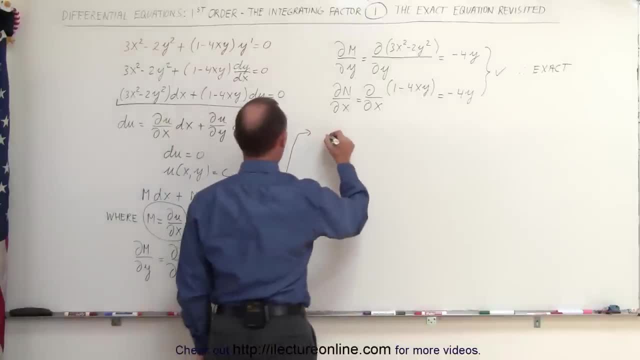 relationship right here and say that the partial of u is equal to m times the partial of x, and so therefore u would be equal to the integral of m times the partial of x, plus some function of y, because in this case we know that y is a constant. so we know that y is a constant in this case. 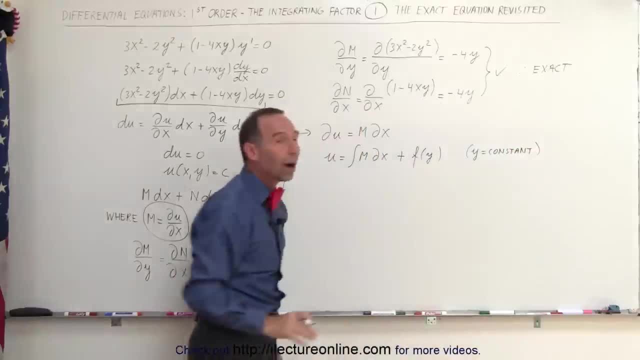 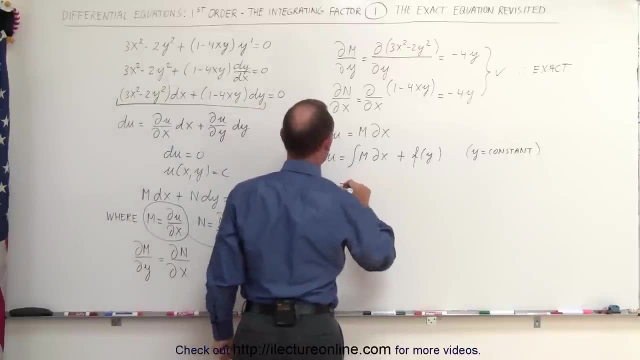 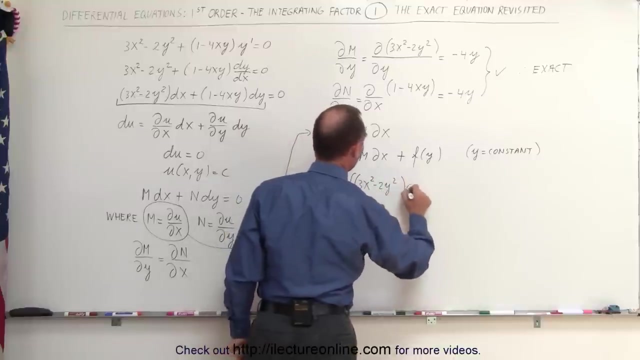 and so we know that we can end up with some function of y, because y, in this case, is a constant. so m, in this case, is equal to this quantity right here. so this would be the integral of 3 x squared minus 2 y squared with respect to x. only that means, in this case, y is a constant. well, so we're going to have 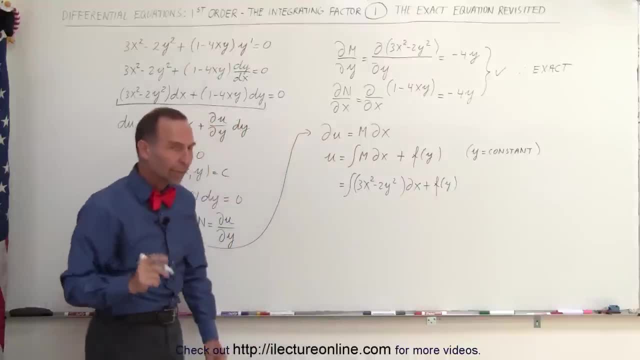 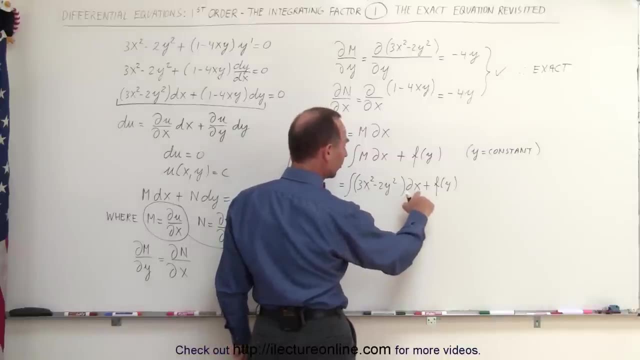 some function of y. take the integral of that, we get the following. we get: u is equal to, that would be 3 x. oh, that would be. since it's respect to x, it would be 3 x cubed over 3 minus 2 y squared x. because of. 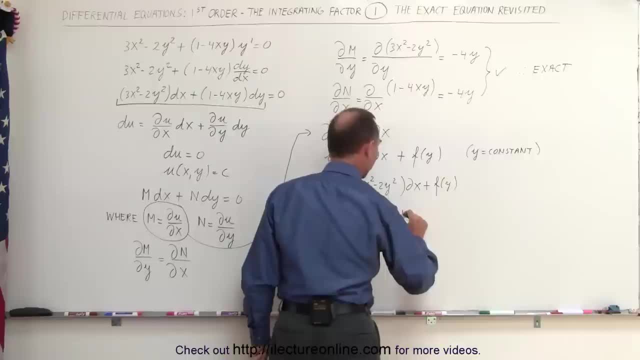 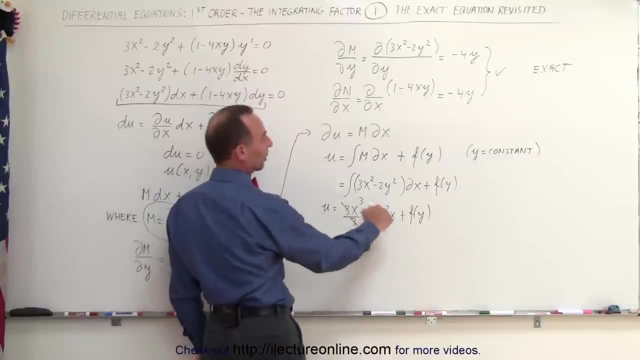 course, minus 2 y squared would be constant and that would be plus some function of y, of course, the three scan slots. that leaves us with u equals x, cubed, minus 2 y squared, x plus some function of y. now we can do the same with the other relationship. we can do the same with this. 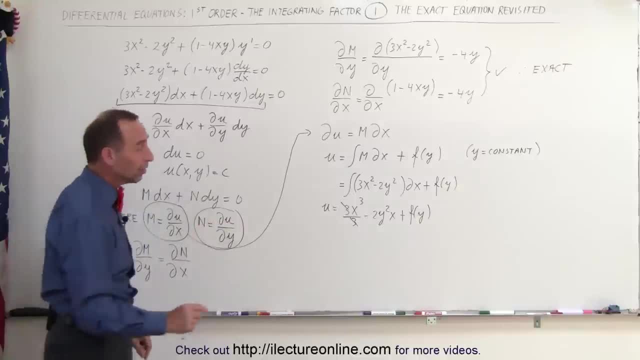 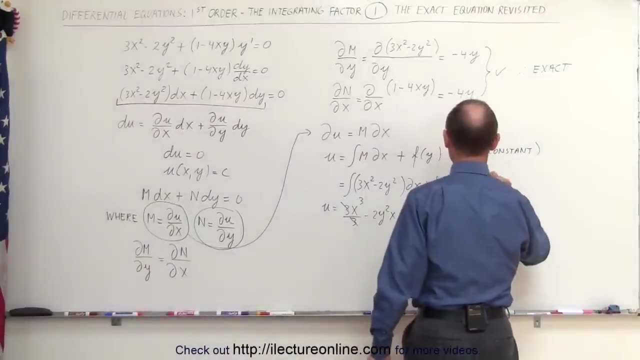 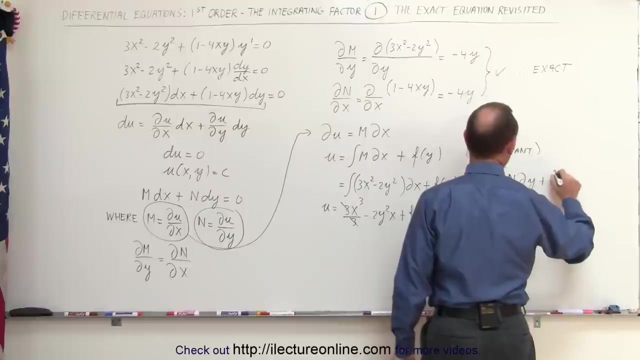 relationship we can also solve for u, and the reason i want to do that is because we can do the same, because i don't know yet what f of y is equal to, so i'm going to do it again with this relationship. say that u is equal to the integral of n times the parcel of y plus some function of x, because 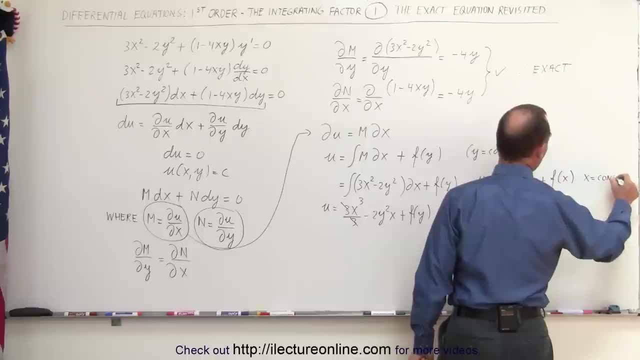 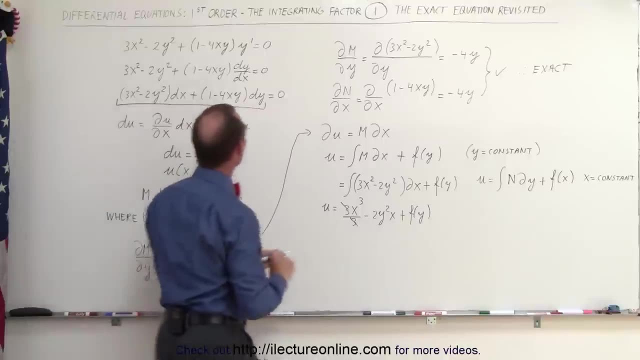 in this case we know that x is going to be a constant like. so then we plug in what n is equal to remember. n was this quantity right here. so 1 minus 4 x y. so this is equal to the integral of 1 minus 4 x y. so this is equal to the integral of 1 minus 4 x y. so this is equal to the integral. 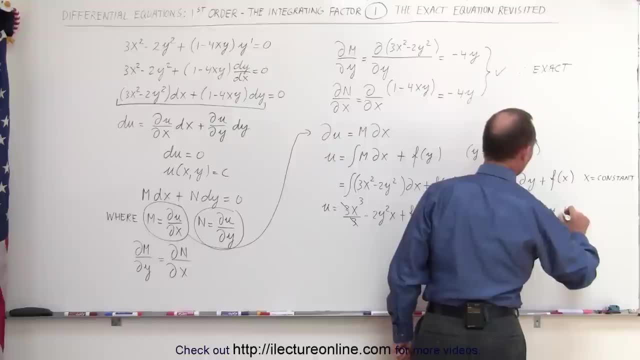 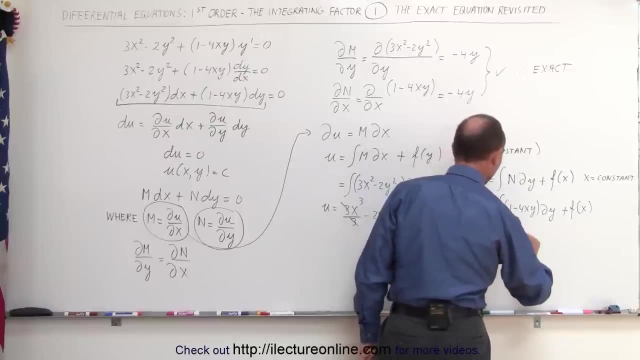 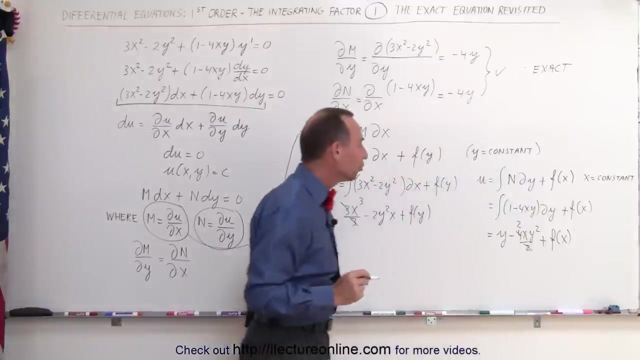 of x- y with respect to y being the variable, plus some function of x, and so this would be equal. to integrate this, you get y minus. so we get 4 x- y squared over 2, minus 4 x- y squared over 2, plus some function of x. of course, this and this cancels out, so we get y minus 2 x- y squared plus. 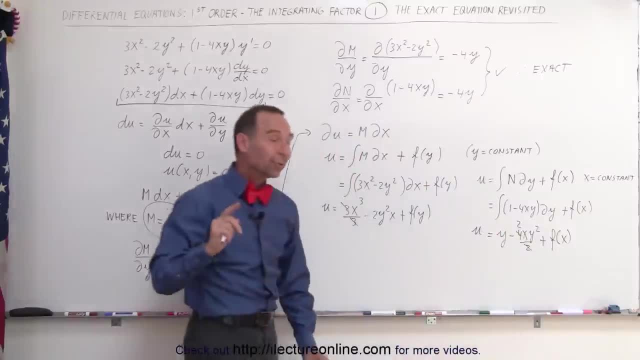 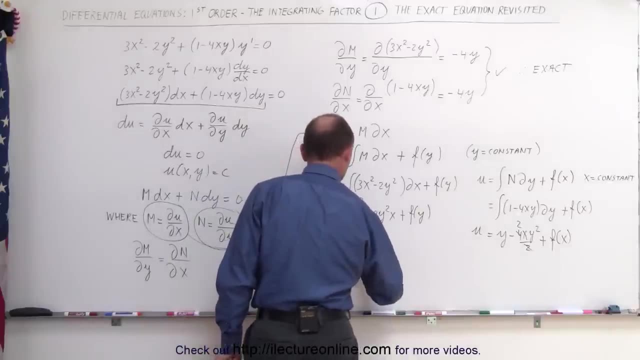 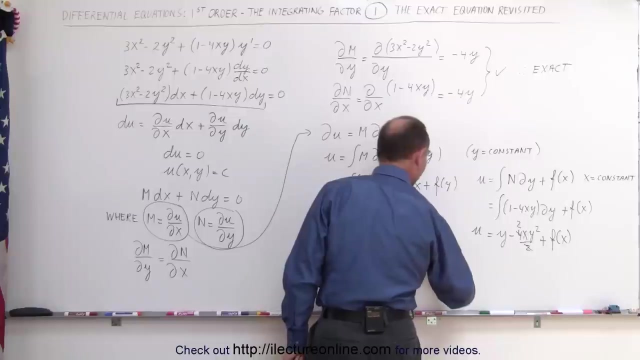 f of x and of course this is also equal to u. and then if we said these two equal to each other, because they must be equal to each other, then we get x cubed minus 2 y squared. plus some function of y must equal y minus, that would be 2 x y squared. 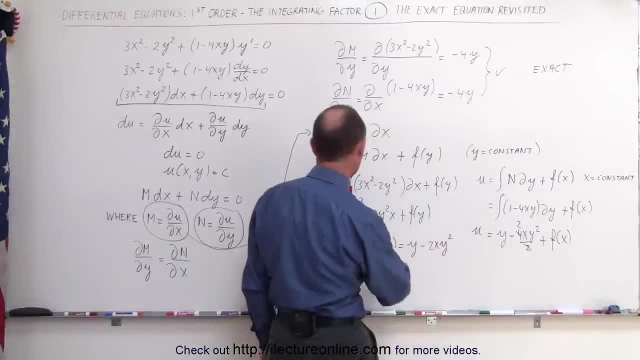 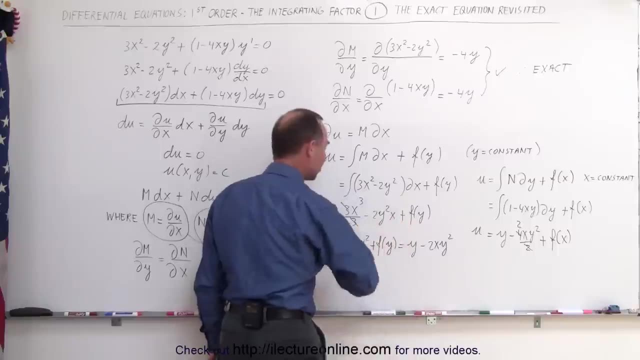 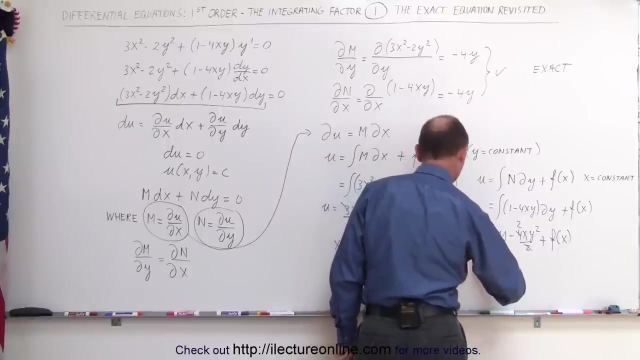 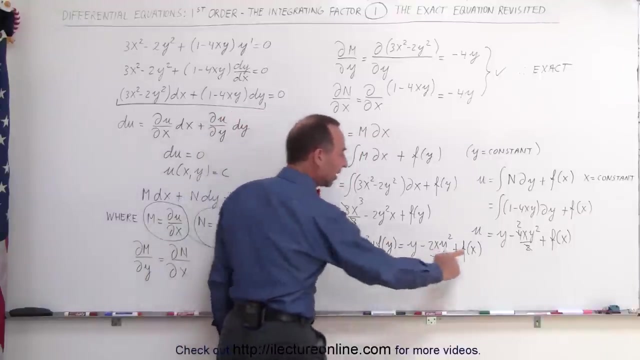 oh, i'm missing something here. ah, here i forgot my x. i didn't copy my x down over here, so otherwise that cannot be equal. so because i have minus 2 x, y squared here plus some function of x, notice that this here is equal to that on the left side. i have an x cube on the right side of an. 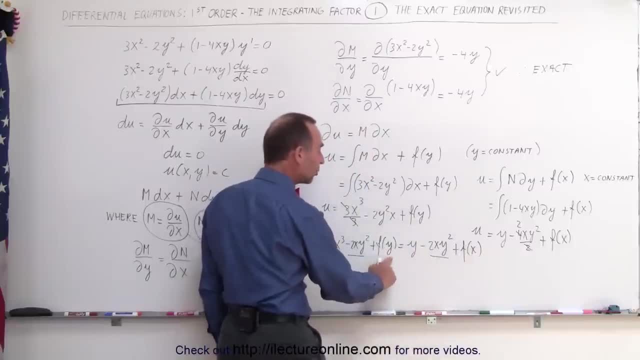 function of x on the right side. i have a y in the left side of a function of y, which means that the function of y is equal to y and the function of x is equal to x cubed. so therefore, my solution then is that u is equal to x cubed minus 2 x squaredangan careers, but w is non-frequency medium of z, so this is: 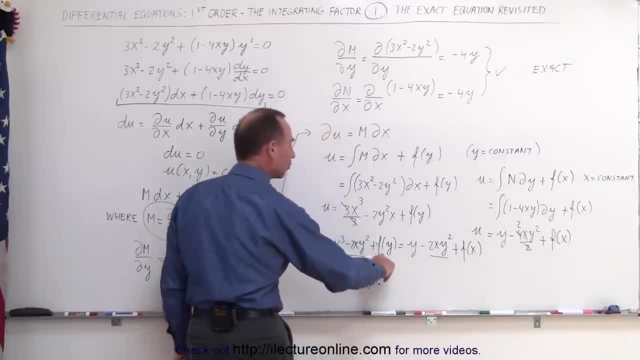 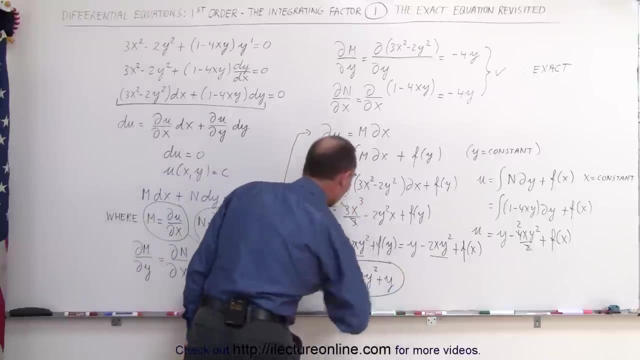 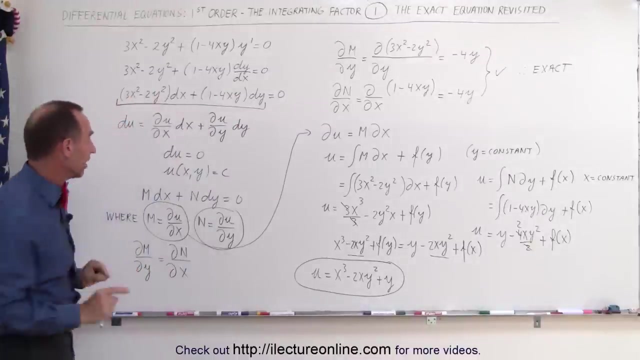 i think transitioning over to u Drive Adjusting. So another function, aka one of these solution of x can be one of x, y squared, and this function of y has to be equal to y, so it would be plus y. so this is then the function u, of which the du is equal to my differential equation, and since I know that, 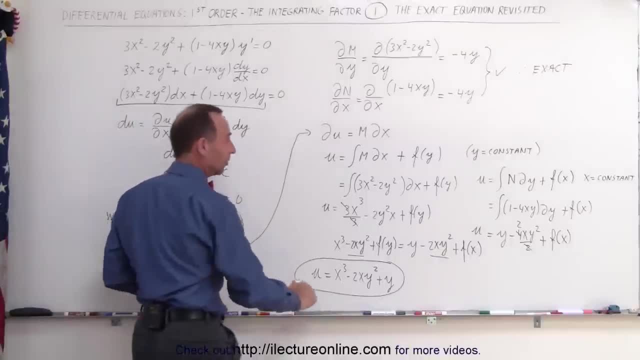 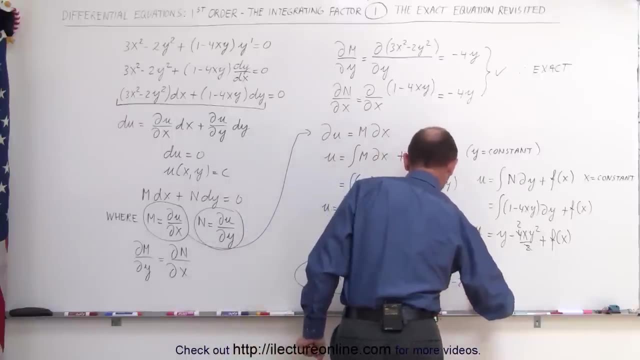 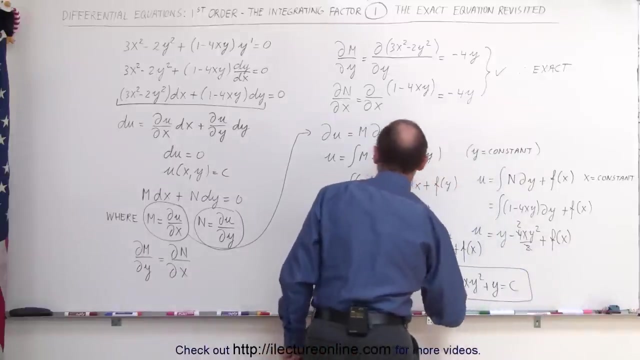 u is equal to a constant, I can set this equal to a constant and therefore I can say that the solution can then be written that x cubed minus 2, x, y squared plus y must equal a constant and therefore this is the solution to my original differential equation, because the differential